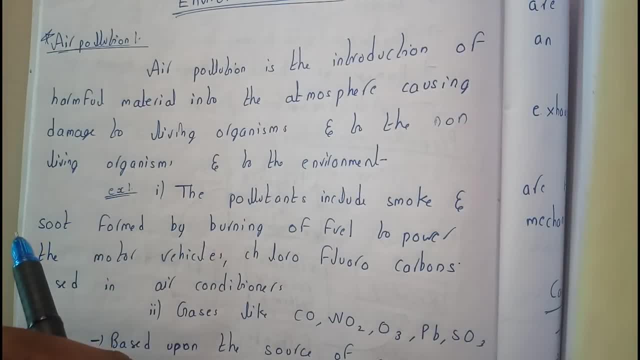 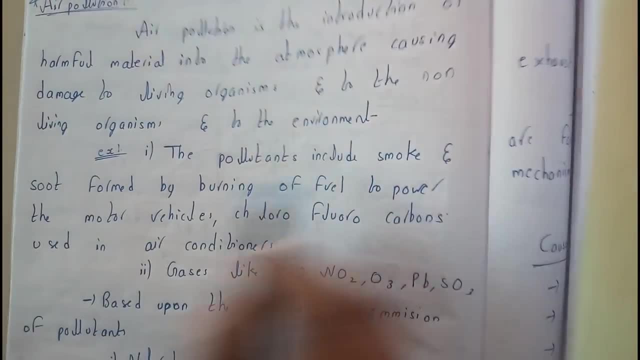 but exemption of dangerous gases. it includes and many other things. Let us take some examples of air pollution. which causes air pollution? The pollutants include smoke soot formed from fuels. While we are burning fuels or anything, we will be getting a smoke right. 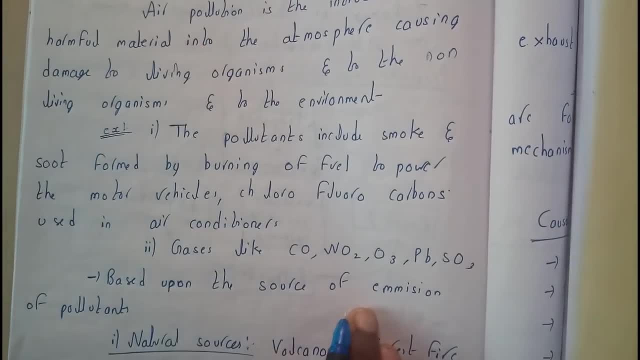 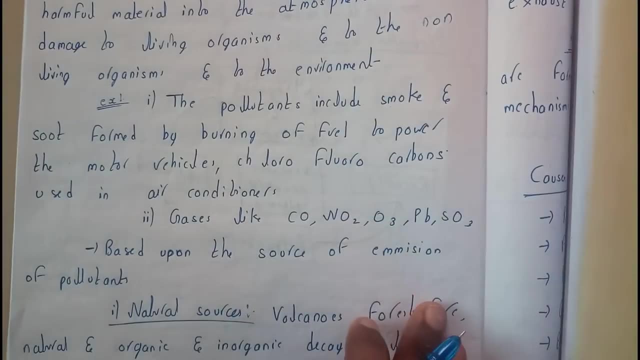 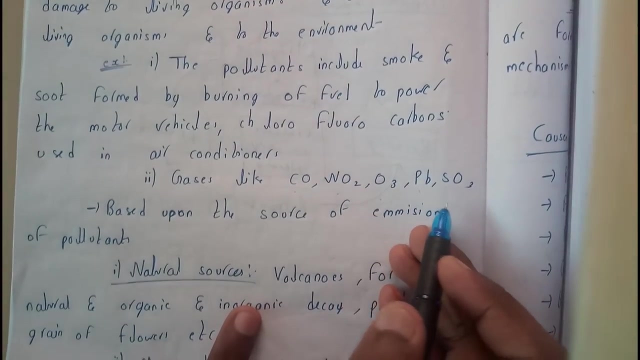 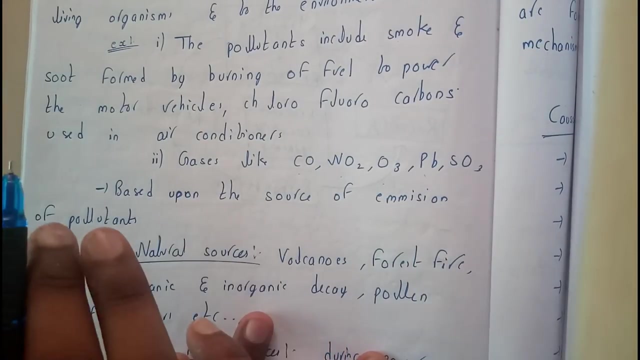 That we will be calling as soot And chlorofluorocarbons that are used in our air conditioners, And there are many gases which cause air pollution, such as carbon monoxide, nitrogen dioxide, ozone, lead and SO3.. Based upon these emissions, I hope up to now everyone got a. 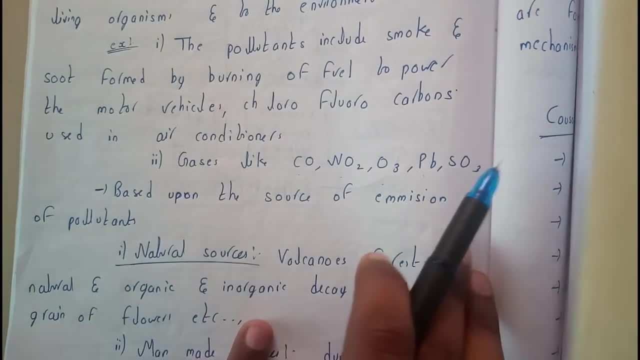 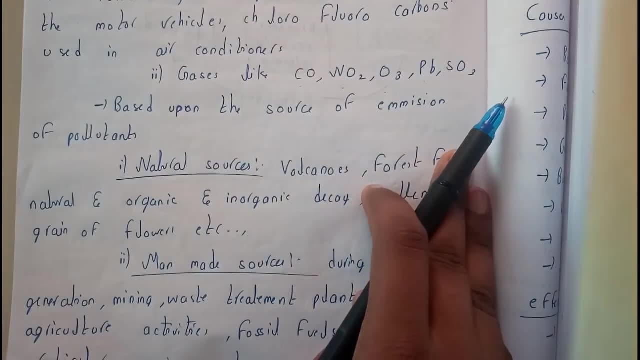 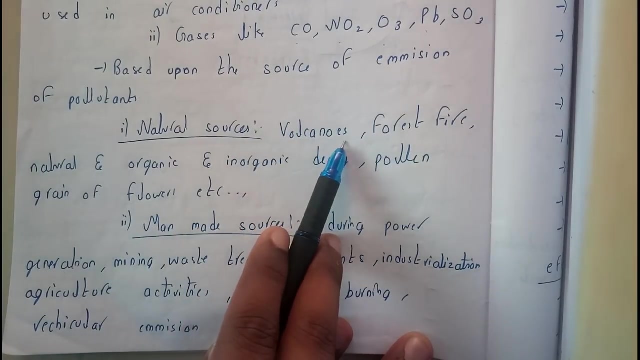 sense of what caused the pollution. according to researchers, There are few natural causes, thing likeRCs and man made sources Which, growing up, are nothing but volcanic eruptions, forest on fire due to high temperature, natural and inorganic decay and pollen grams from flowers. 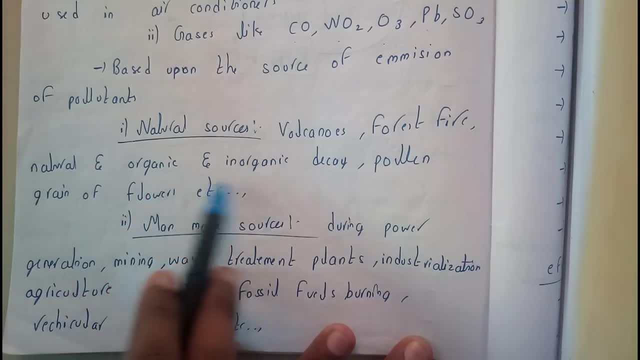 Today I am going to discuss natural and inorganic decay examples: Inаж tai kato yag, roma, уп, Coca Cola, Jyoti, Cap, Psychiokin, etc. Fuel – 3 triv, konkretemabilitatee diluting the soil for 24 hours a day. 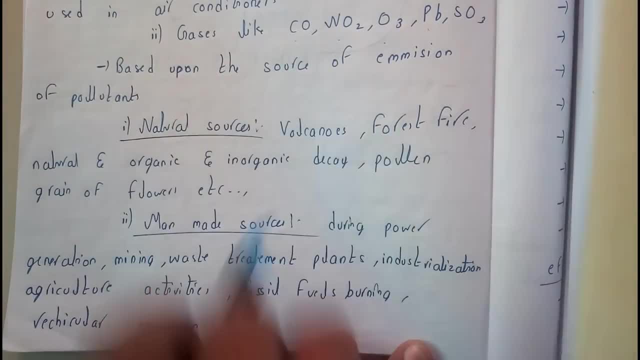 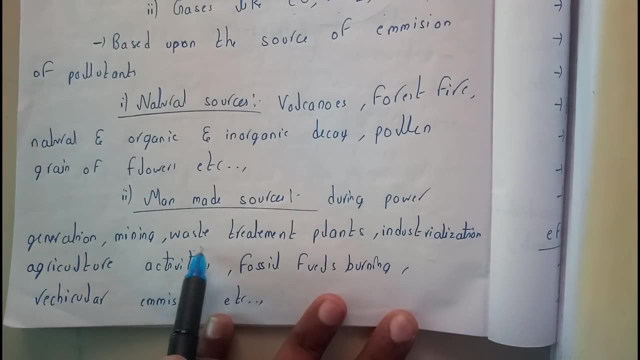 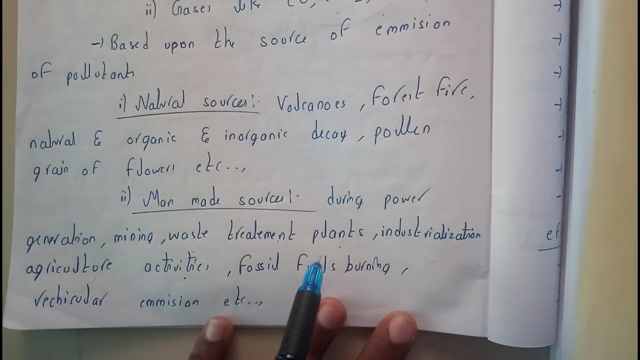 Tree ignition of ganska high water content would probably indeed cause water mínimo. these are the basic natural ways of air pollution. when we come to man-made- man-made during power generation, mining, waste treatment of plants, industrialization, agricultural activities and burning of fossil fuels and vehicular assumption emissions- these are the main causes. 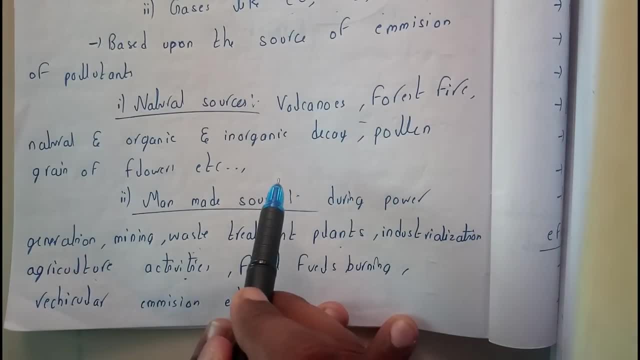 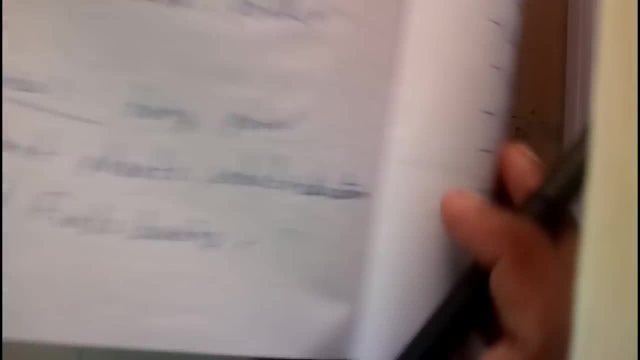 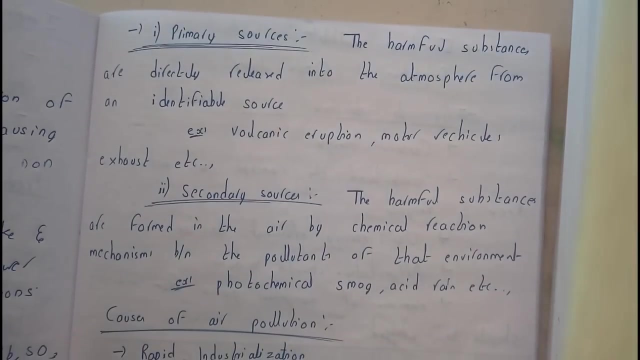 by human, and these are the main causes by nature. i hope everyone got an idea on sources of air pollution, so let's go further into sources of air pollution. sources of air pollution are furtherly divided into primary source and secondary source. okay, basically, what is a primary and what is it? 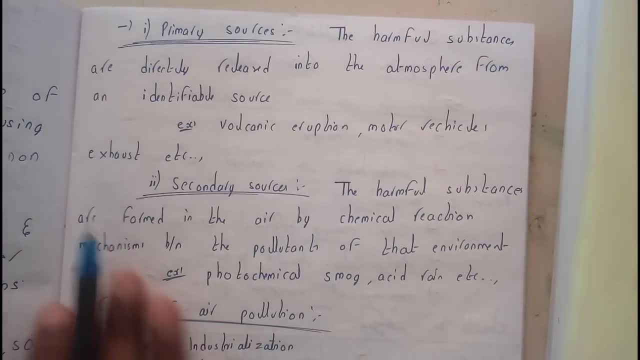 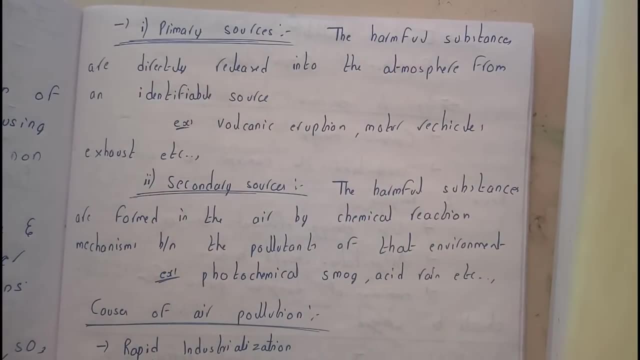 we'll be going through them in depth, don't worry guys, it's really easy. okay, basically, primary sources are nothing but the primary sources of air pollution and the secondary sources of air pollution, but they are directly released into the air, something like some dangerous gas from an. 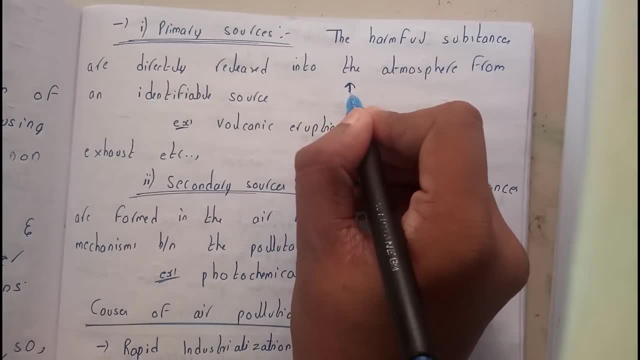 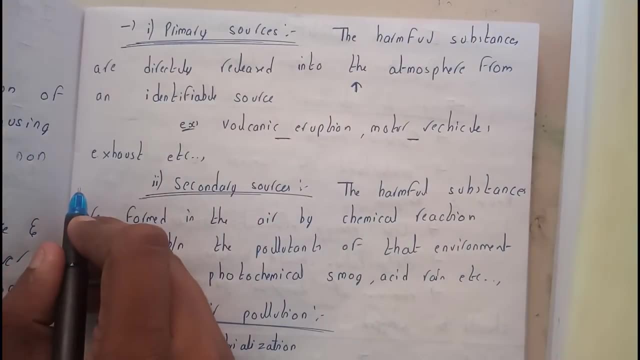 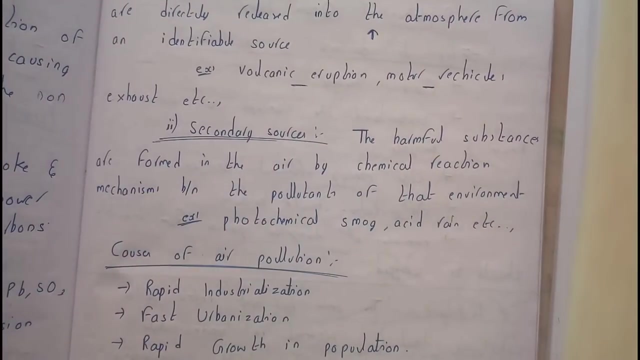 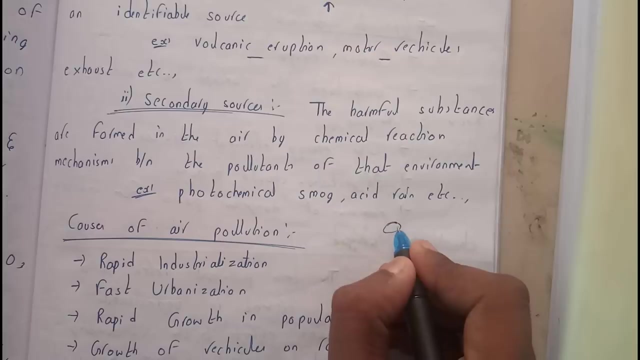 industry is directly released into the air which causes air pollution, such as volcanic eruptions, motor vehicles, okay. and whenever we come to the secondary sources? secondary sources are that, even in this, the gas or something is emitted out which causes air pollution, this gas initially combines with another gas to form the danger- danger to air you are discussing. 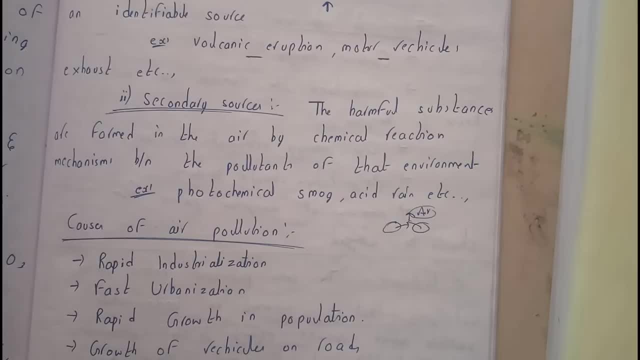 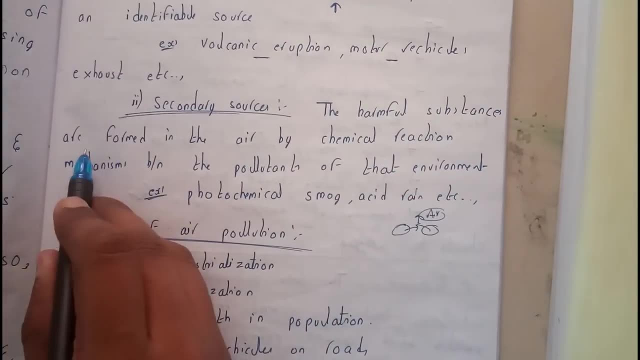 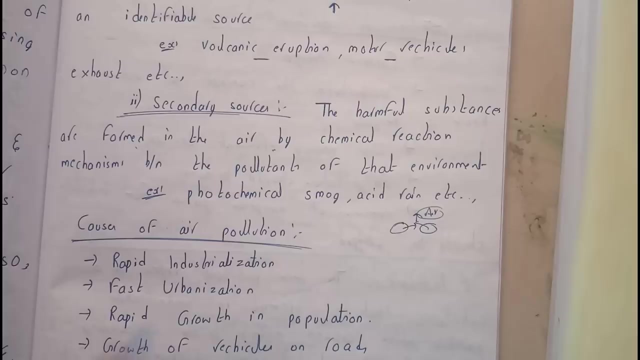 about air pollution, right? so these two mix up to form a dangerous thing, or a dangerous composition or chemical to form air pollution. so the harmful substances are formed in air by chemical reaction mechanism between the pollutants. i hope you understood what i am saying. okay, example will be photochemical smoke and acid. 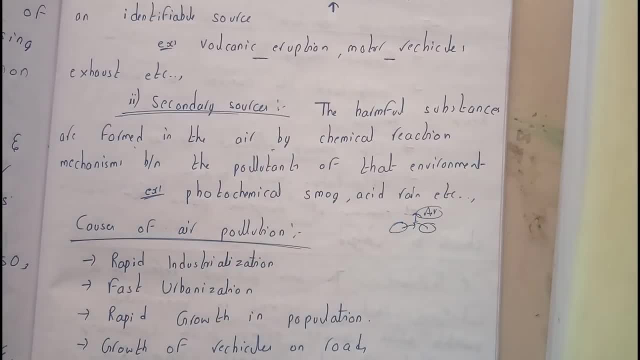 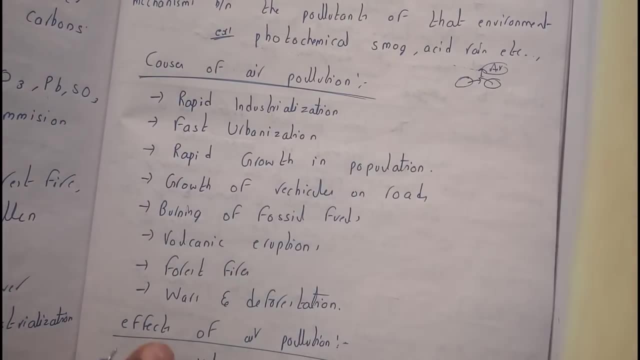 rain. i hope everyone knows about photochemical smog and acid rain. okay, we'll not go in depth in them, that's fine. okay, up to now, we have discussed what is air pollution and what are the causes and sources of air pollution. okay, let us go through causes of air pollution now. 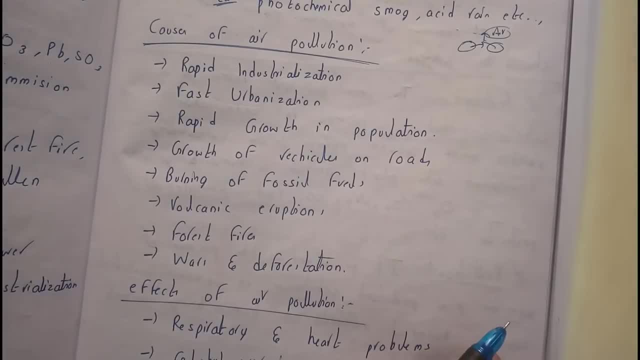 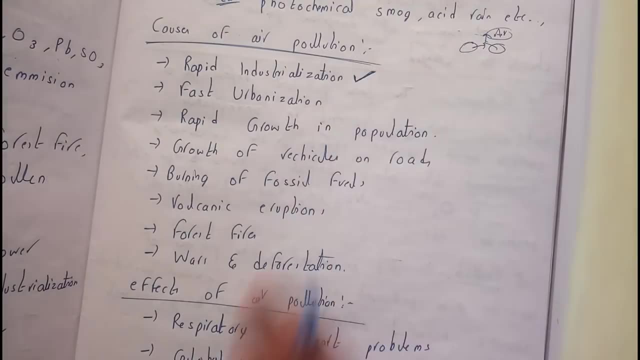 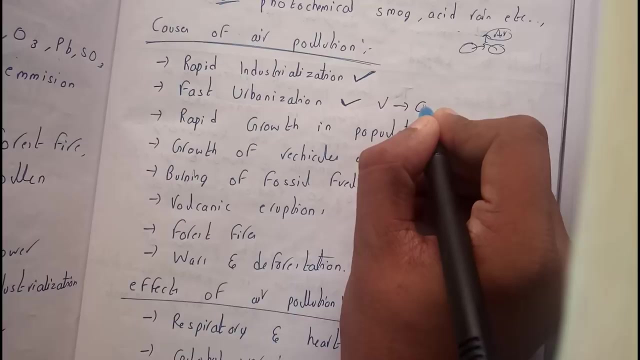 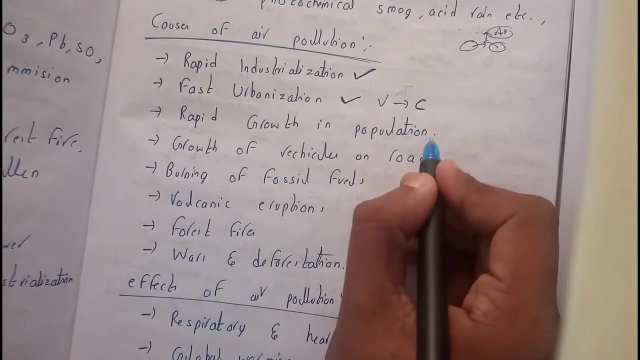 so causes of air pollution? okay, one of the major cause is rapid industrialization, as the number of industries increases, pollution increases, and fast urbanization. urbanization is nothing but villages to cities, development of villages into cities, which increases industrialization, which increases growth in population, even growth in population causes, as growth in population leads. 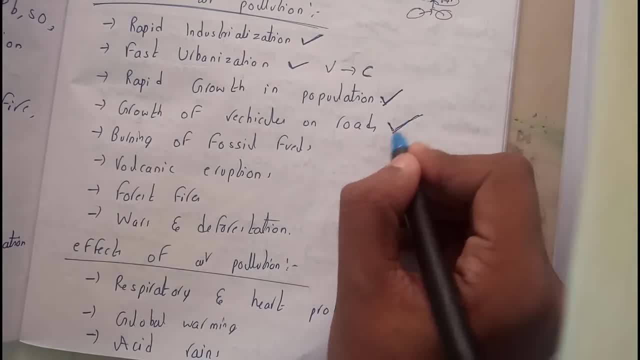 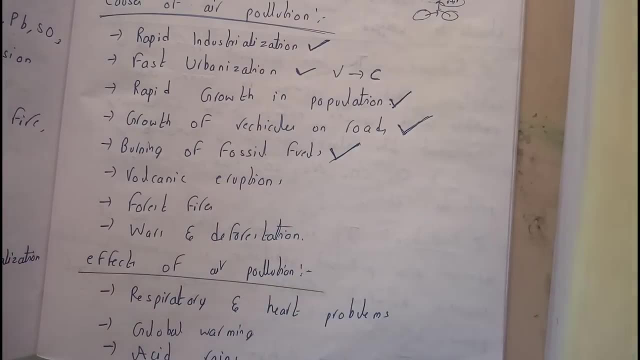 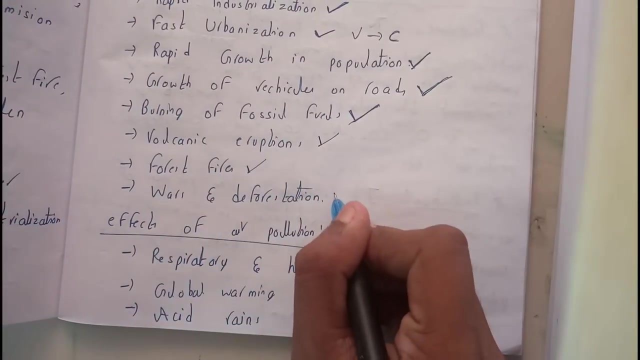 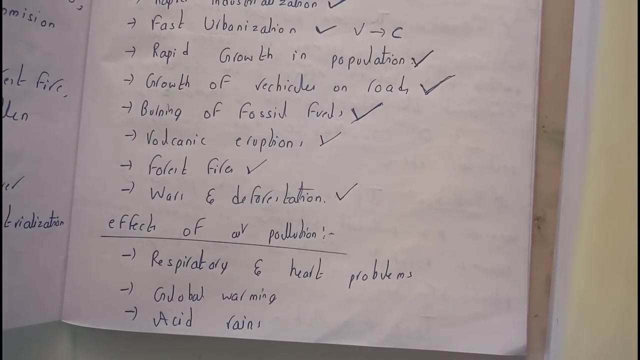 to vehicles on the road. increase in vehicles on the road, increase in vehicles in the road on the road, increases to consumption of fossil fuels and even volcanic eruptions are also causes. i have just discussed them. forest on fire also, and war and deforestation. these are all the causes of air pollution. and if he particularly asks for: 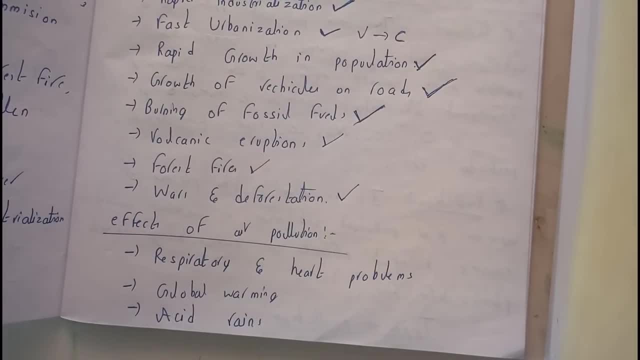 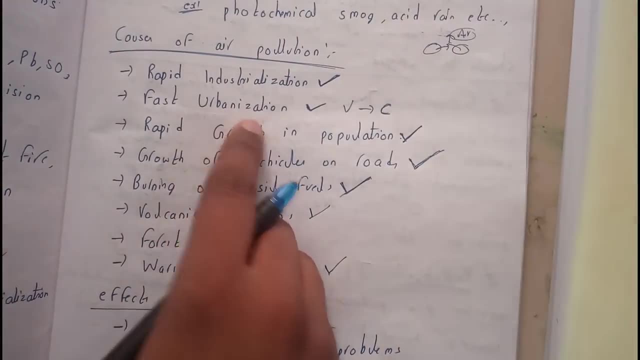 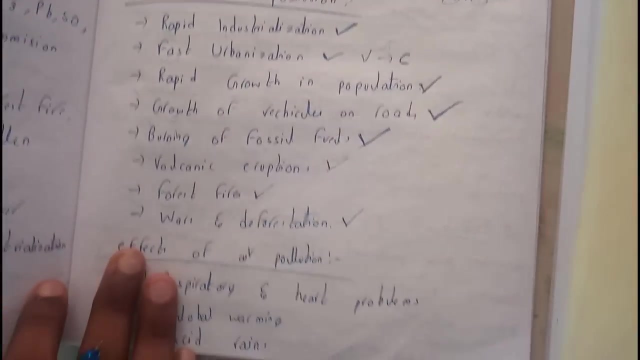 causes of only air pollution. you can just write the definition and write the name and just a small reason: industrialization, as the industries increases, pollution increases, urbanization, change of villages to cities, like that. you need to just make small, small sentences so that your answer will be elaborated. okay, i hope everyone is clear up to now, so let's go through. 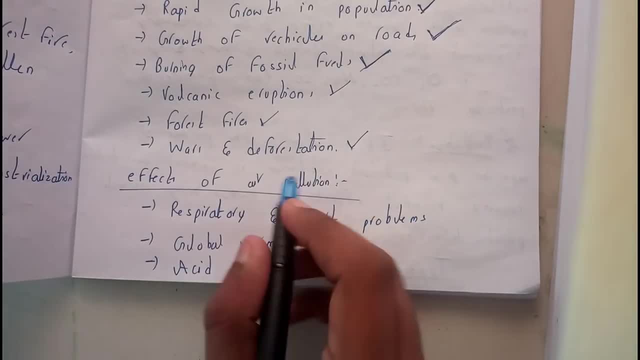 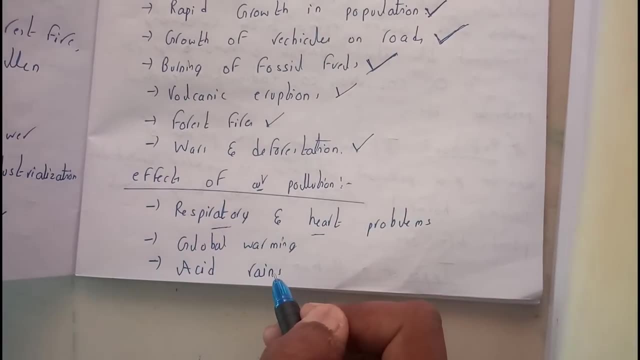 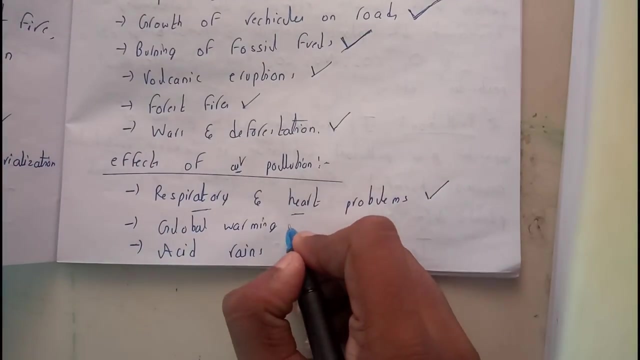 effects of air pollution. okay, the polluted air if we inhale we're gonna get respiratory problems and heart problems. okay, i hope everyone is clear up to now. and these gases, if they are dangerous gases. that forms global warming and it causes acid rain. also, acid rain is nothing but. 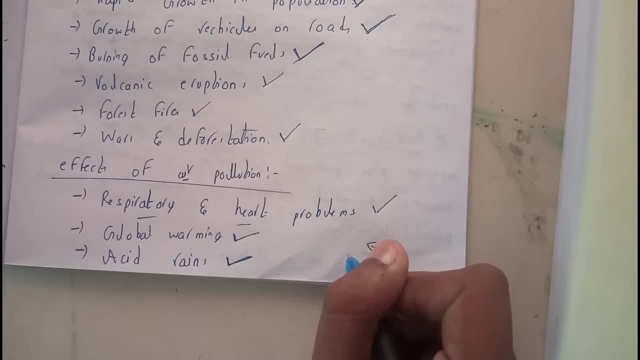 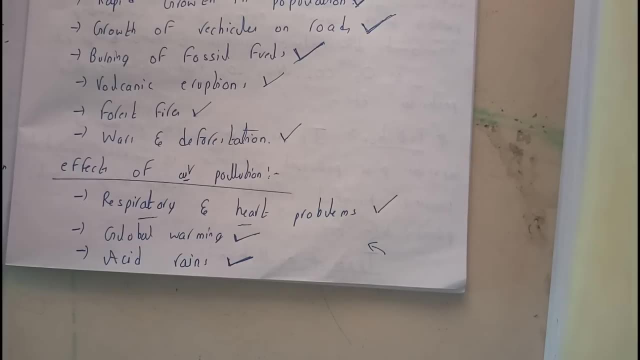 addition of some gases to the water vapor. water vapor or clouds, that's, it mix us with them, with those gases, and it forms acid like nitric acid, sulfuric acid. like that. it will be forming some acids and it falls as rain, which is very, very dangerous. so air pollution is the reason for 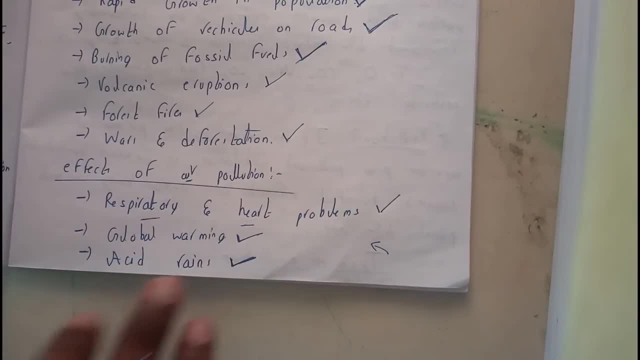 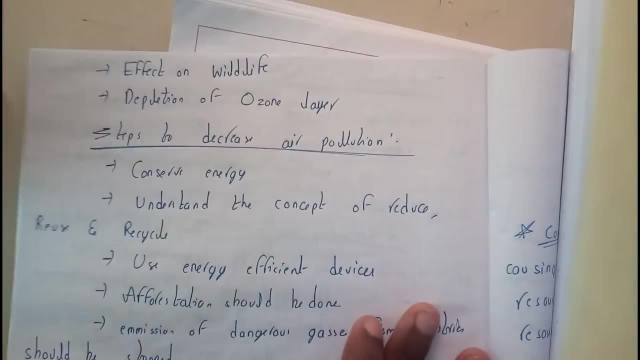 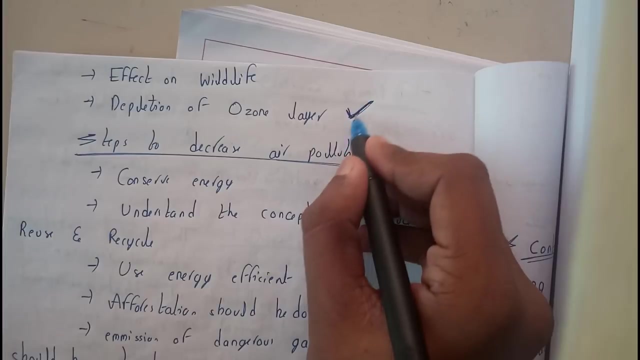 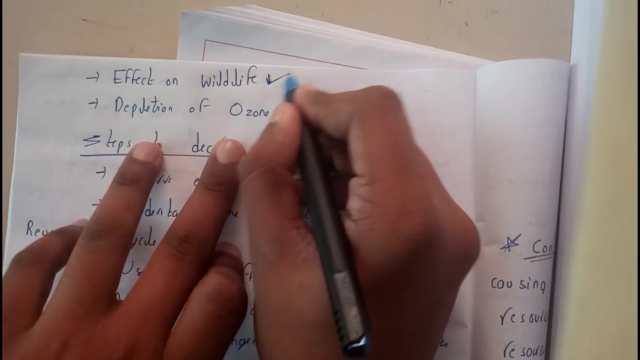 acid rays, global warming and respiratory and heart problems. okay, and it is also responsible for it is responsible both for depletion of ozone layer- one is familiar with ozone layer. okay, even it is depleted by air pollution- and it also affects wildlife. okay, guys, you can write many reasons. guys, in our daily life only we'll be seeing many. 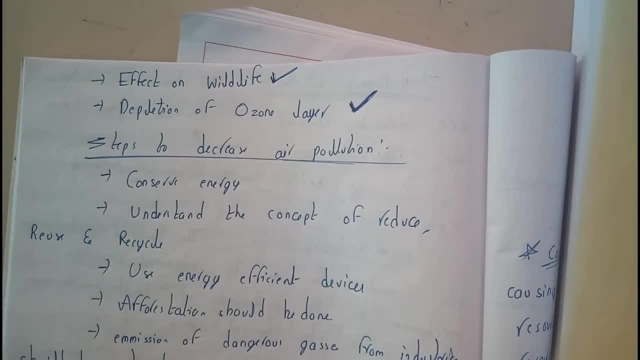 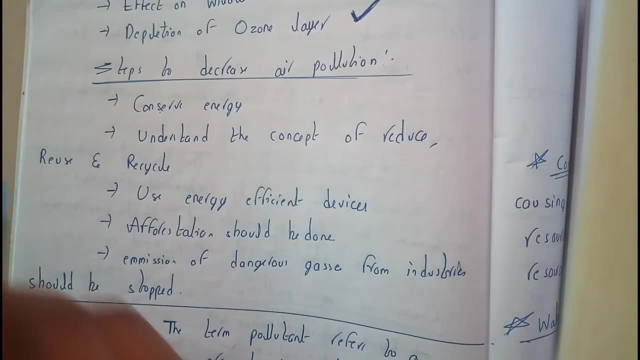 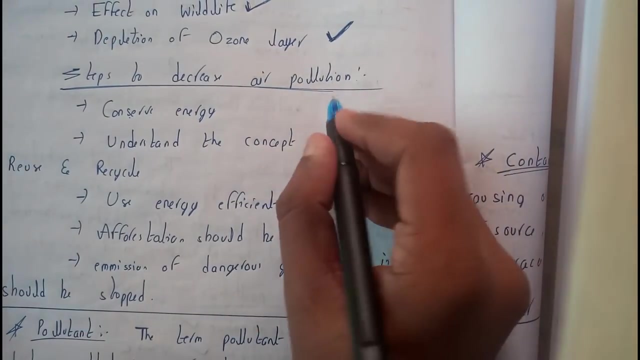 reasons. what are the effects of air pollution? okay. what are the steps to decrease air pollution now? okay, we need to conserve energy. yes, that's true, because we are as if in our daily life. if there, if there is a family, they will be having two to three cars, and there will be even there is a. 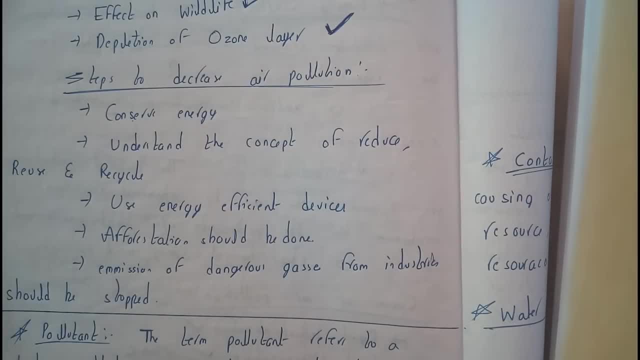 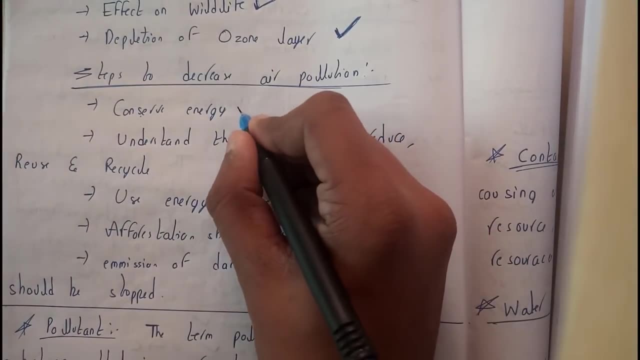 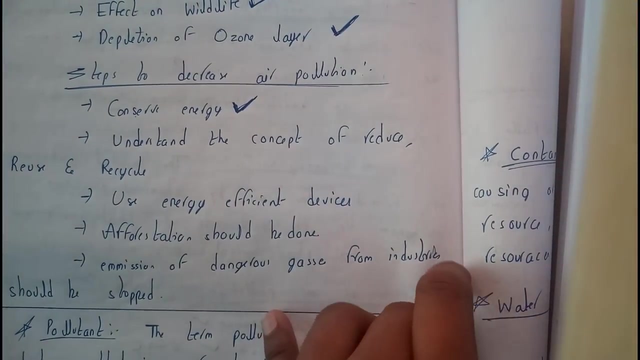 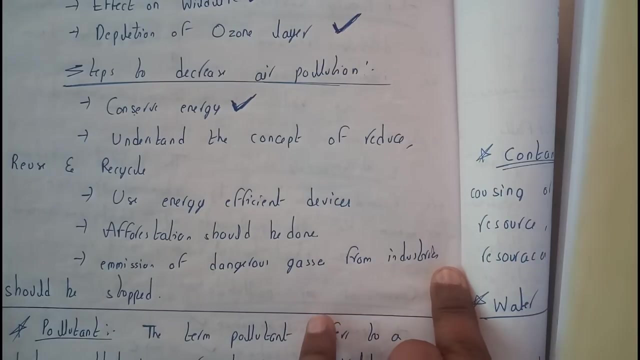 single guy going out, he'll be taking the car that causes a lots of pollution. a car can cause a lots of pollution, so conservation of energy is really, really important. even it comes under electrical energy. also, while producing the electrical energy, there is a lots of pollution. even by using coal will be getting an ash at the end which is of no use, so we need to conserve the. 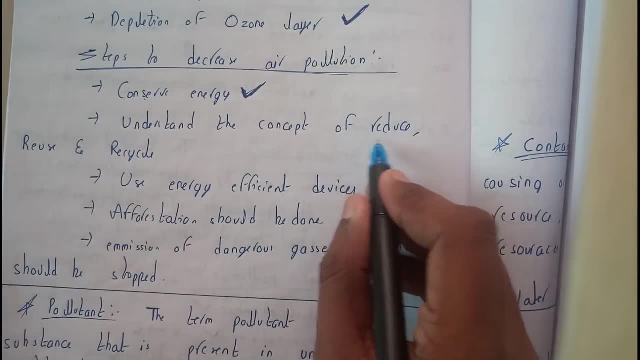 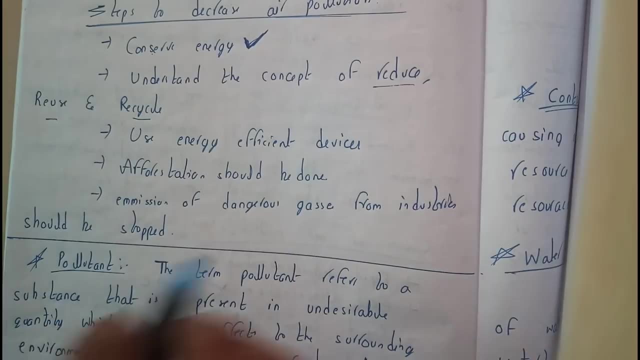 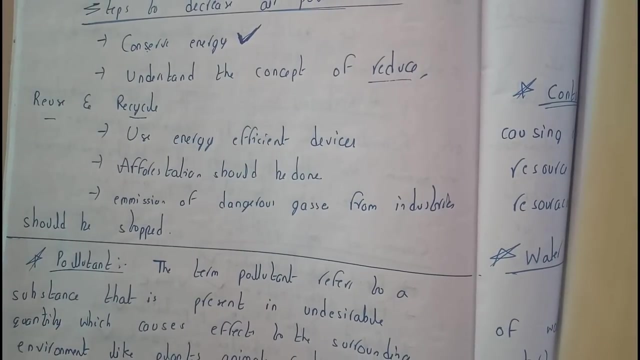 energy. we need to follow the rules like reduce, reuse and recycle. I know everyone- we are, every one of us- we will be using plastic bags which cannot be reused, which cannot be recycled, which causes the lots and lots of pollution. so try to use paper bags and we should use the